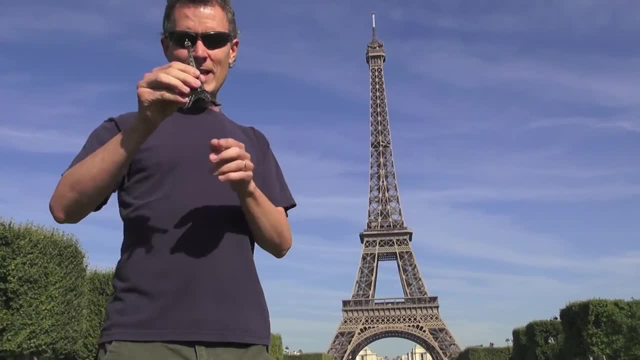 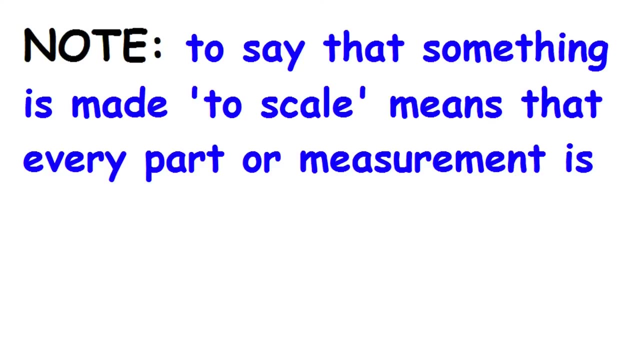 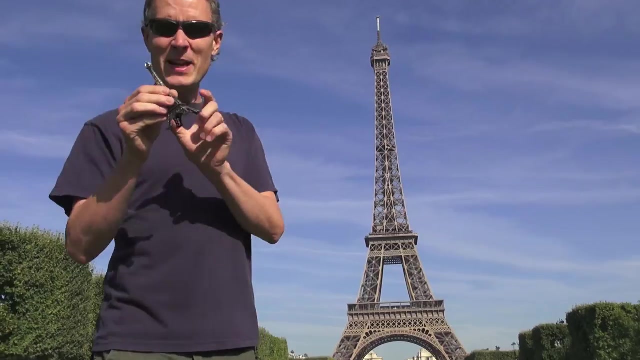 this is a reduction. We know it's sort of to scale. To say that something is made to scale means that every part or measurement is multiplied or divided. It might not be exactly to scale, but we're going to assume that it's more or less to. 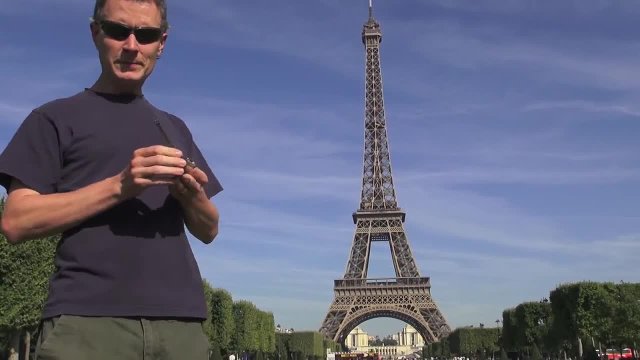 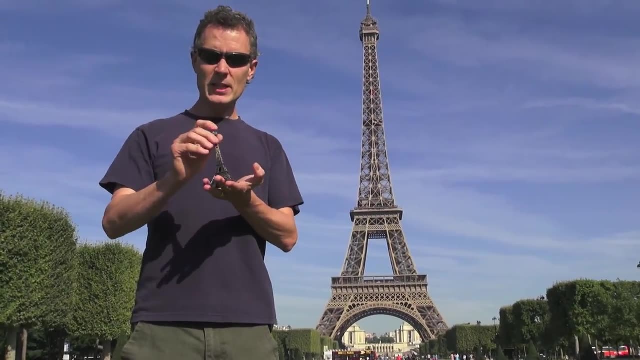 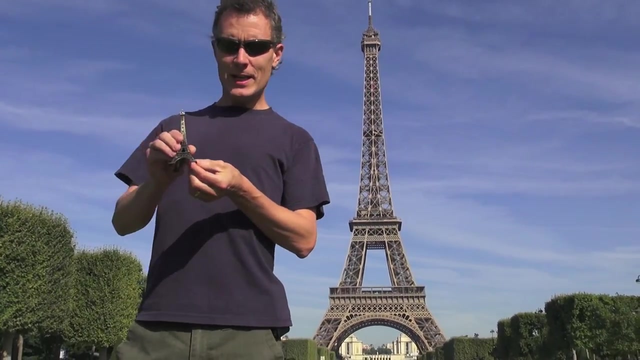 scale. We're going to work out the scale of this model as compared to the real thing. The real Eiffel Tower is about 324 meters tall. This is about 13 centimeters tall. The real Eiffel Tower is about 100 meters wide at the base and this is about 4 centimeters. 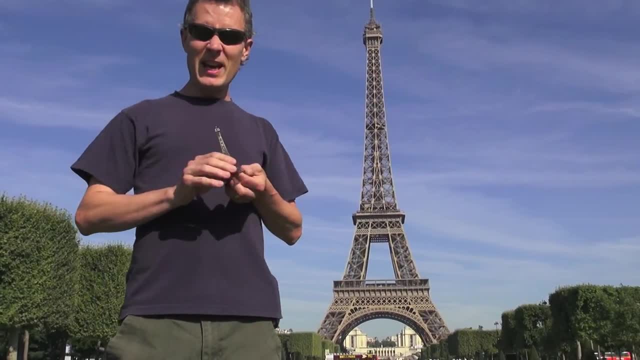 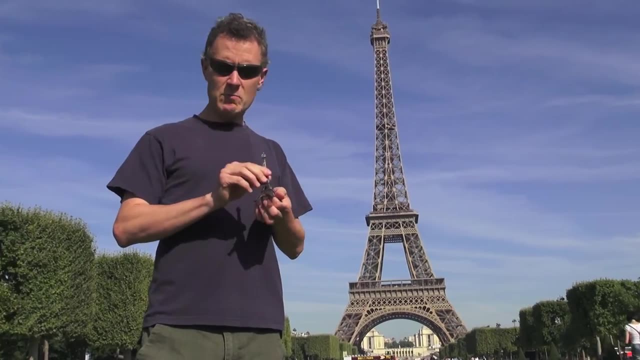 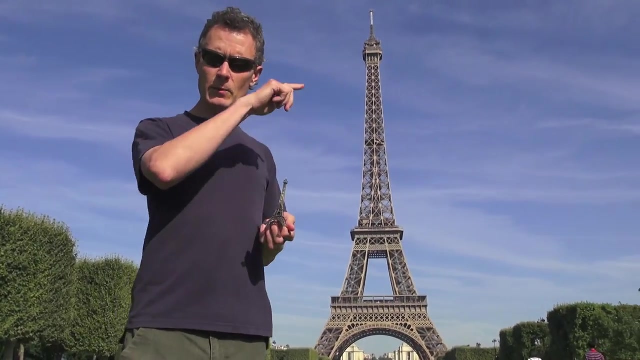 wide at the base. Let's take those two things and see what the scale of this thing is. We'll start with the width. If you want to work out the scale of a model of something, if you take the measurement on the model- 4 centimeters- and you take the actual measurement- 100 meters, and we're 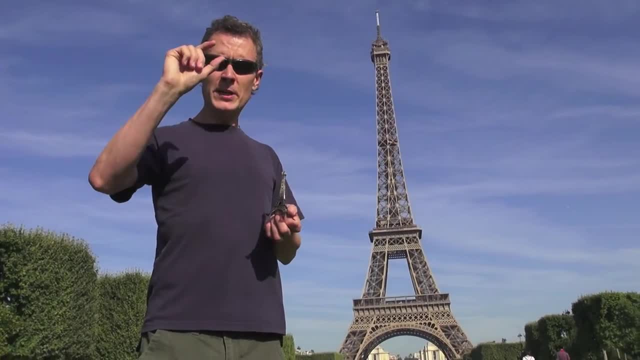 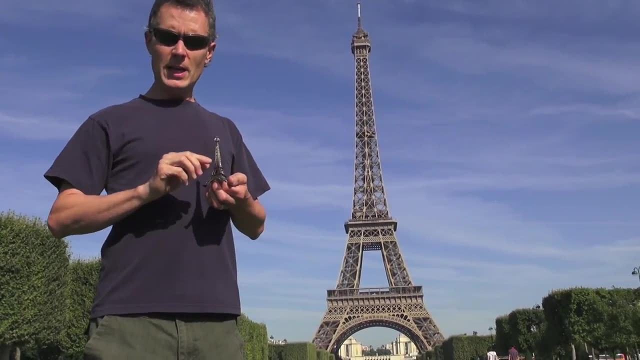 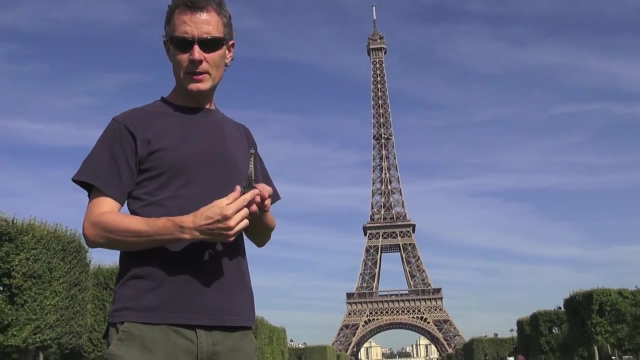 going to divide those two things. So we're going to divide 100 meters by 4 centimeters, But first we're going to change that 100 meters to centimeters so that we're using the same units. The width is like 10,000 centimeters, 10,000 centimeters divided by 4 centimeters. that 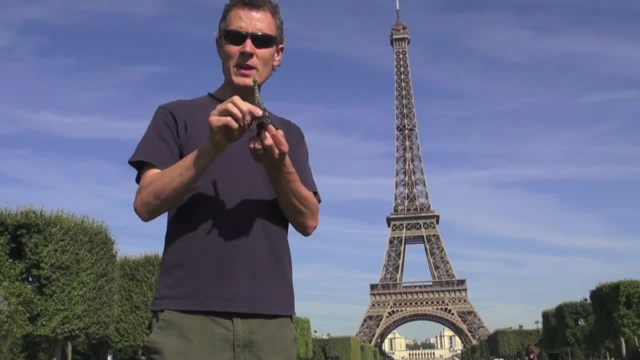 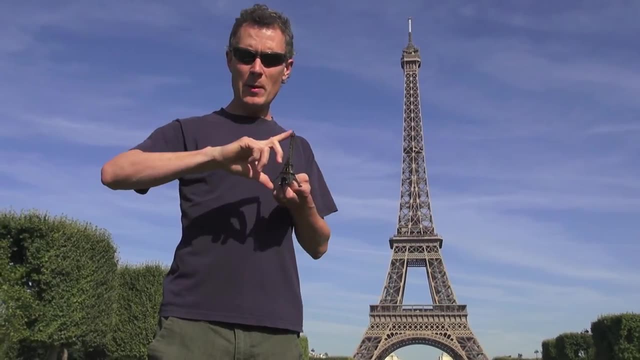 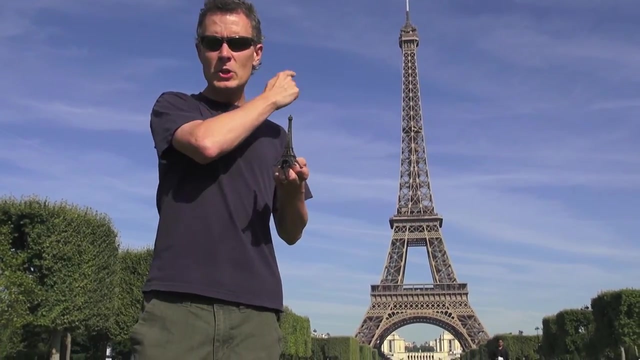 gives us 2,500. So this is about 2,500 times smaller than that. when you look at the base, Or that thing's about 2,500 times bigger than this. Whatever measurement you take on here, if you multiply it by 2,500, you get the measurement on the real thing. 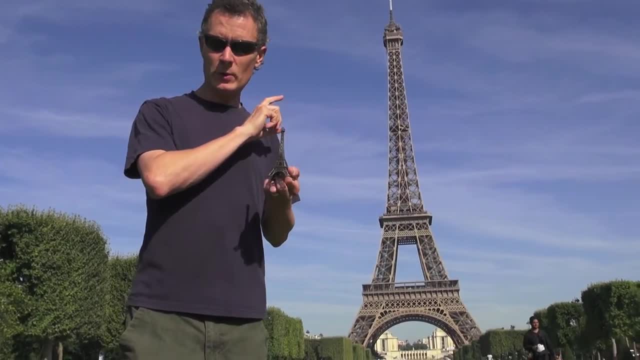 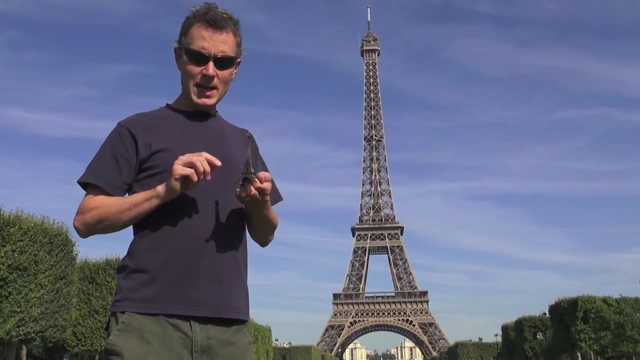 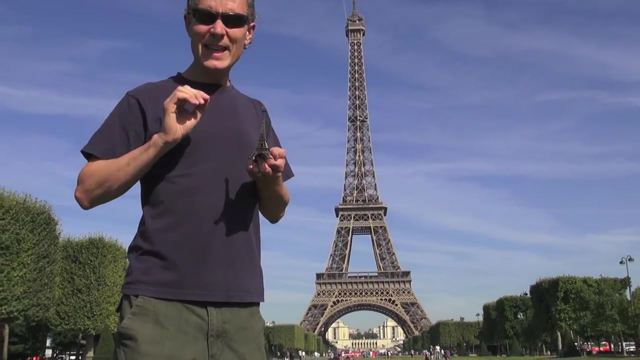 Let's check the height as well. The height of the real thing is about 324 meters, or 322,400 centimeters, And the height of this thing is about 13 centimeters. If you divide those two things, you get approximately, you get about. you get 2,492,, which is about 2,500. 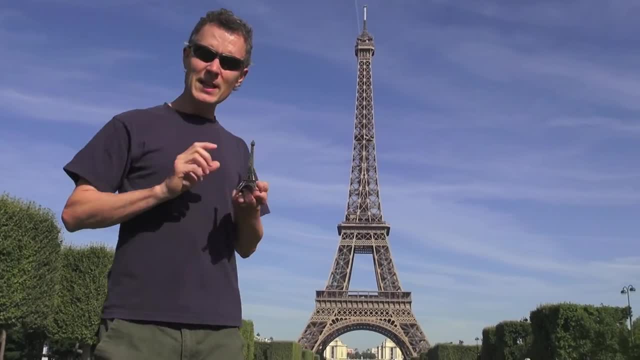 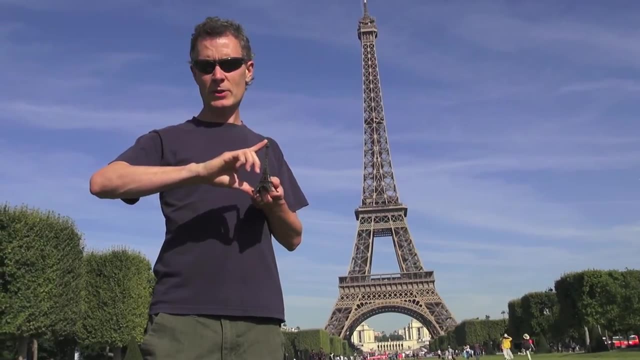 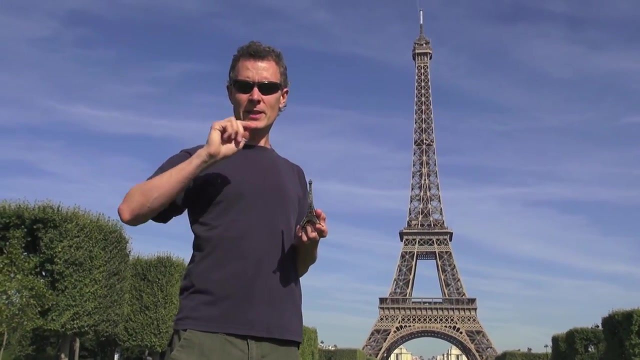 So pretty close. The height and the width are about in the right ratio. The scale you would say then is 1 to 2,500, because this is 2,500 times smaller. If we had a model that was 2,500 times bigger, we would say it's 2,500 to one, all right. 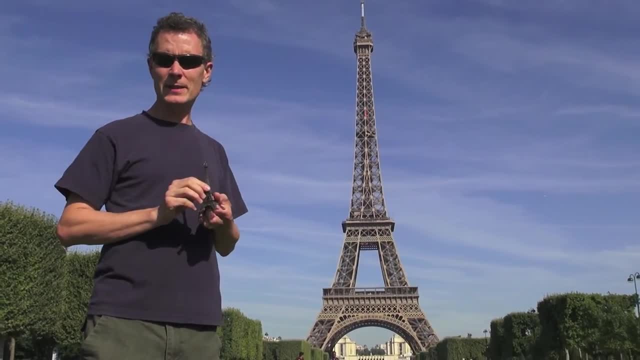 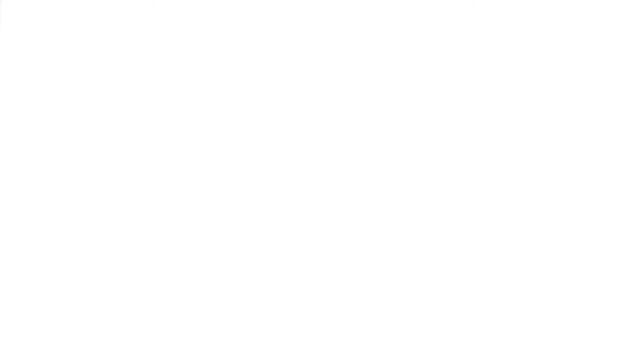 But since this is smaller, it's 1 to 2,500 roughly, All right. So that's the scale of this as compared to the real thing, right there? All right, let's look at it quickly in writing here: what I just described as I was holding. 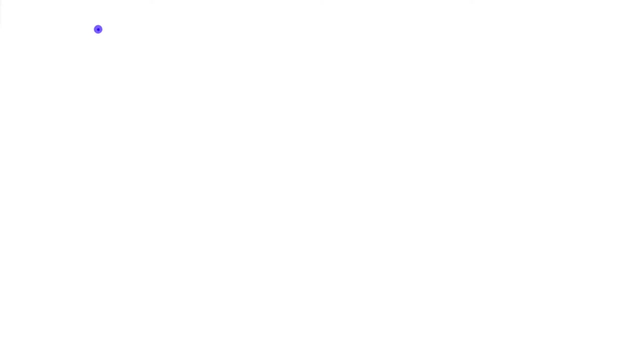 up the model. When you want to figure out the scale of something, you need to compare on the model or or the diagram to a measurement on the actual object. so we first compared the widths. we had four centimeters on the model represented a hundred meters in reality. we need them to be the same unit if we're gonna write. 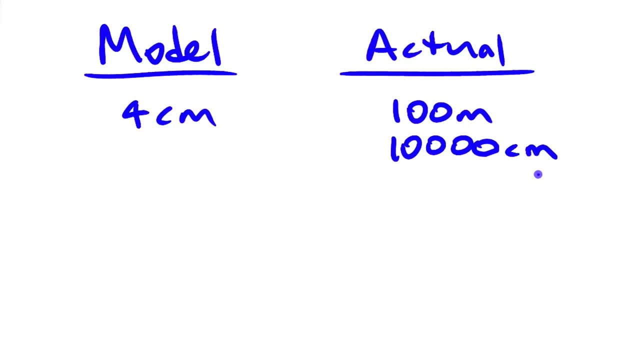 a ratio. so we thought of this as instead 10,000 centimeters. compare those two things. we had four compared to 10,000, but usually you write the. you write the scale like this, where one of the numbers is 1. so if you divide by 4, as I, 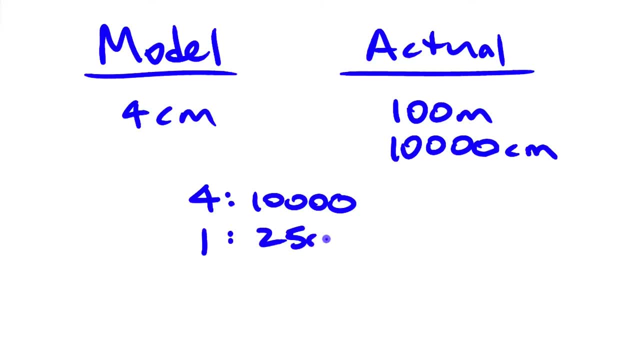 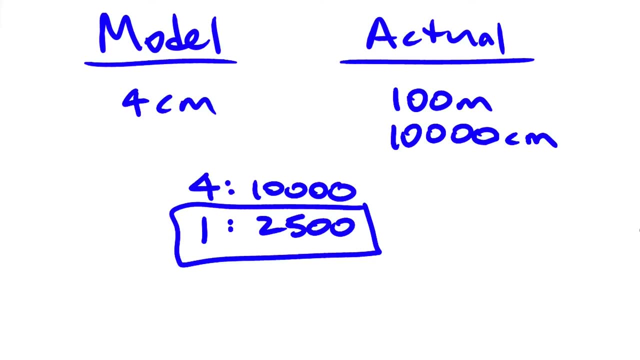 mentioned in the video, you get 2,500, 1 to 2,500. so that's that scale, roughly speaking. now, just as a check, we use the second set of measurements, the heights, and hope that if it is to scale, we're gonna get roughly the same thing here. so 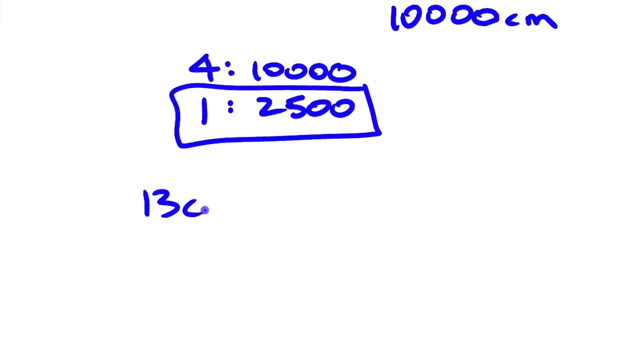 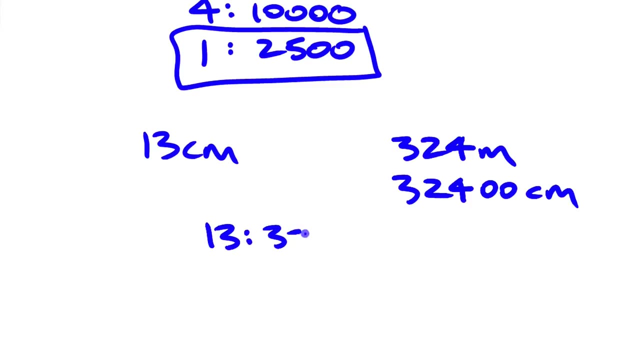 for the heights, we had about 13 centimeters and the actual height 324 meters, or we'll think of it again as 32,000 400 centimeters. when you compare those two- 13 to 32, 4 0, 0- if you divide by 13, you get about, as I said, 2492 here. 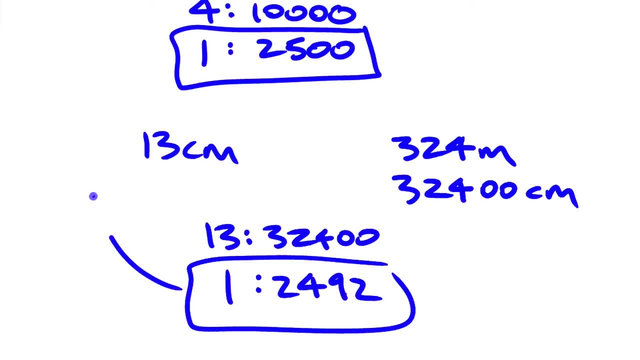 approximately 1 to 2492. that's pretty close right. probably the difference between those numbers isn't because the models, not not exactly the scale. it's probably more likely because 13 centimeters is as accurate as the actual, as accurate as I could achieve in my measurement at the time. so you know. 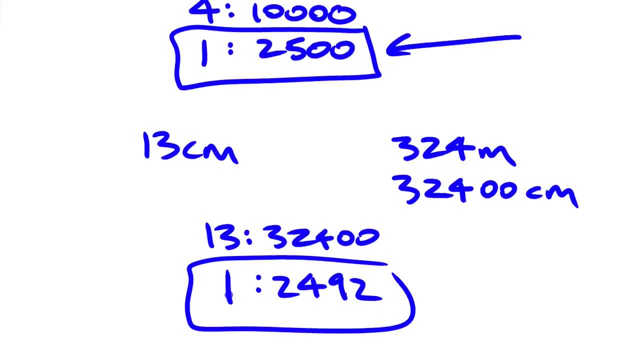 rounding it off, to express what that scale is: 1 to 2,500 is probably about the best you can say again, meaning that one unit on the model corresponds to 2,500 units on the actual thing, the. the model is 2,500 times smaller and if you write, 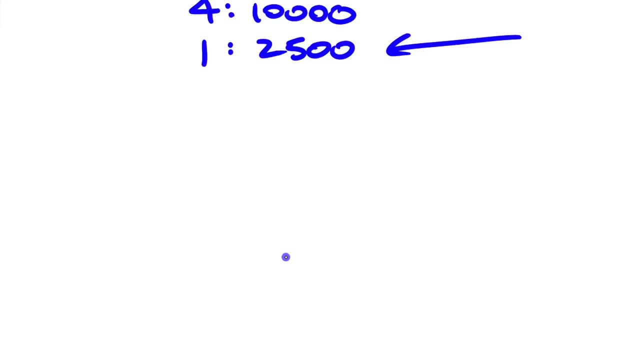 this. sometimes you can write it as a ratio, as a fraction. when you write it as a fraction- 1 to 2,500- you'll probably get less than that, and that's probably the five hundred. like this, it emphasizes the fact that the model is one twenty five. 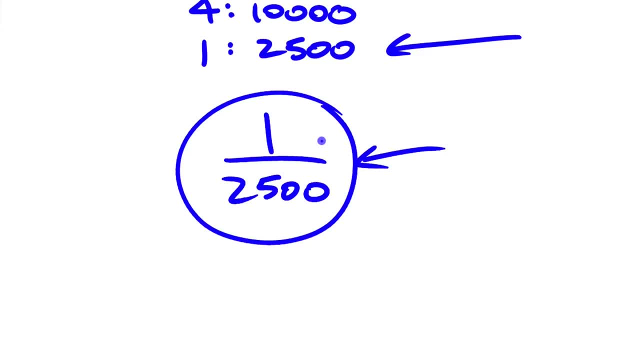 hundredth the size of the actual thing. now, as I mentioned before, if you had a situation where you had a model that was bigger than the actual object, well, this would be turned around. if this were where the model of something was twenty five hundred times bigger, well, that would be the first number here, and that 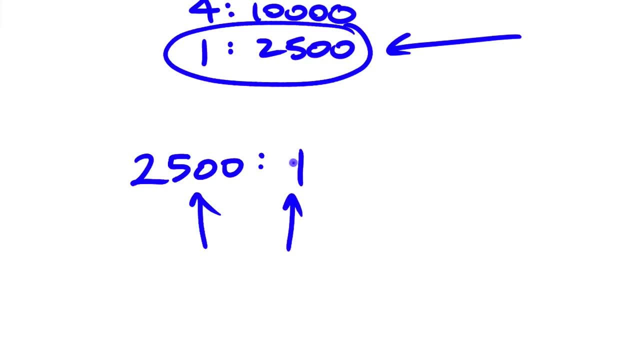 would come second. twenty five hundred to one. when you have a situation where the model or diagram is bigger, then the bigger number is going to be first. right to say that it's twenty five hundred times bigger. you can really see that when you write it as a fraction, because it's twenty five hundred over one or 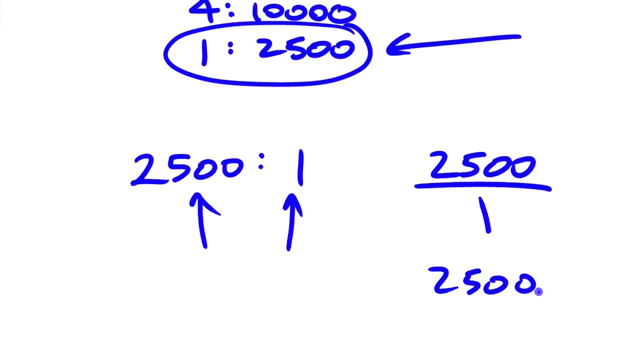 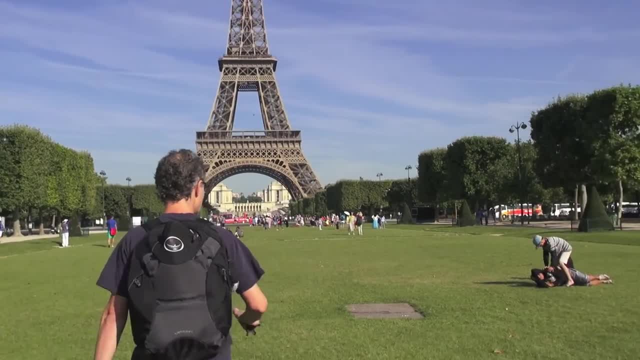 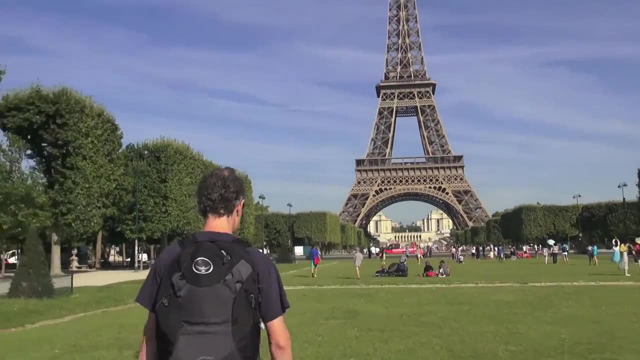 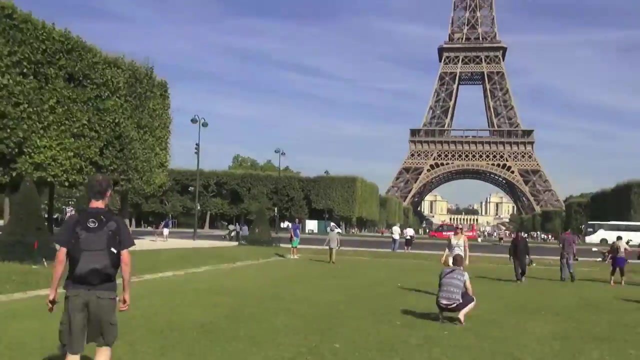 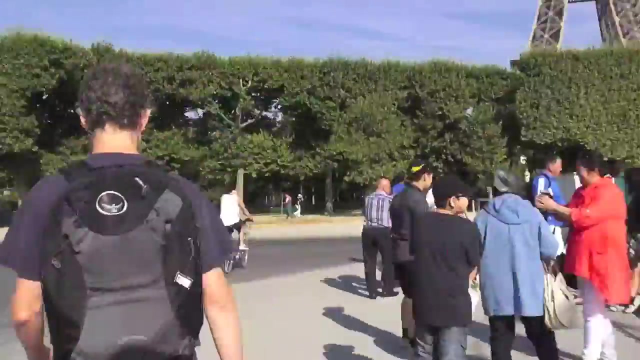 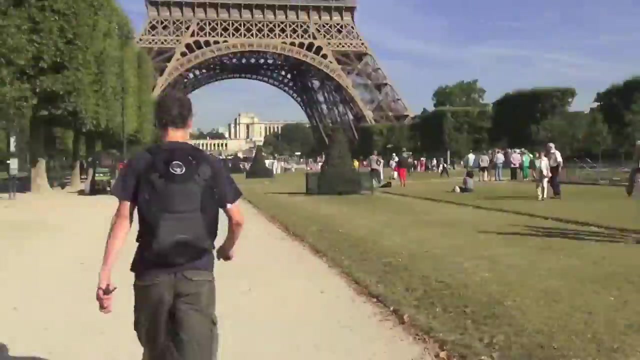 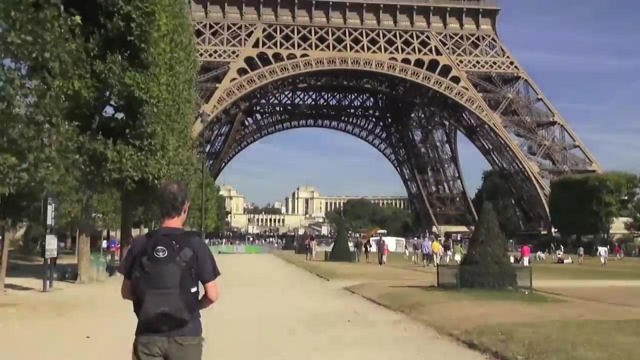 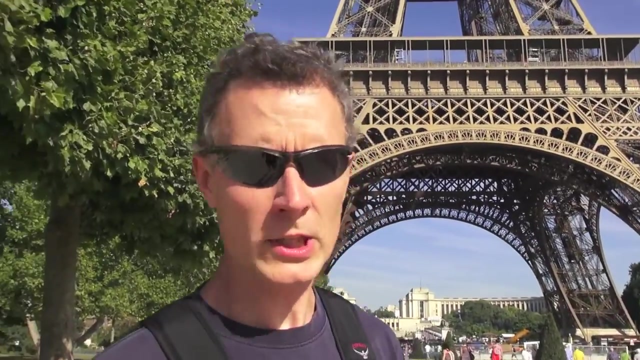 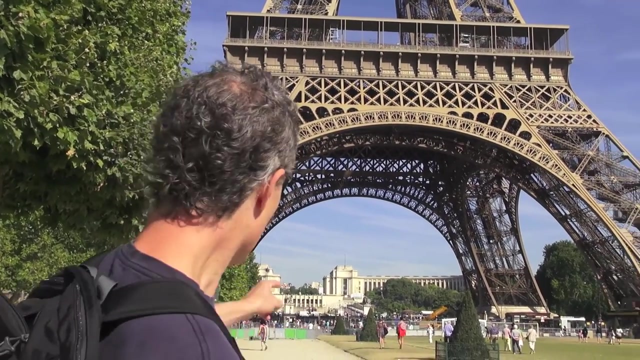 just twenty five hundred, as opposed to the other way, which was one over twenty five hundred. now you know what? before we're done, I think we should go up. we'll get a close look at this thing, you. this is pretty close, it's. it's one of the tallest buildings in Europe. let's go. 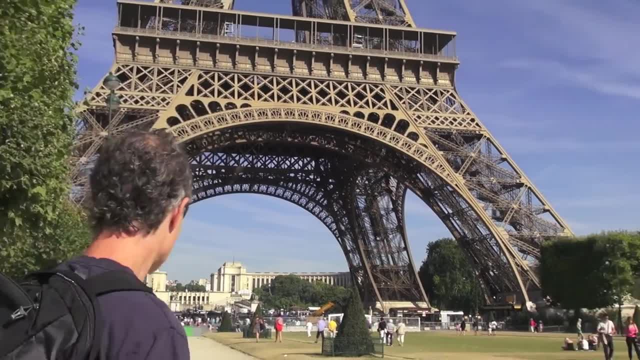 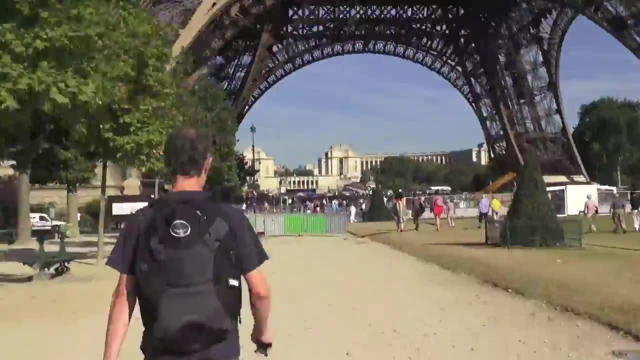 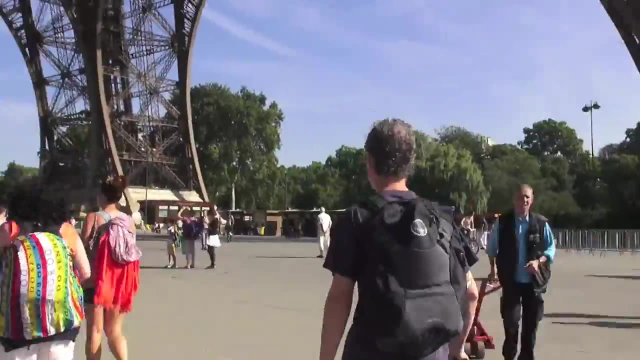 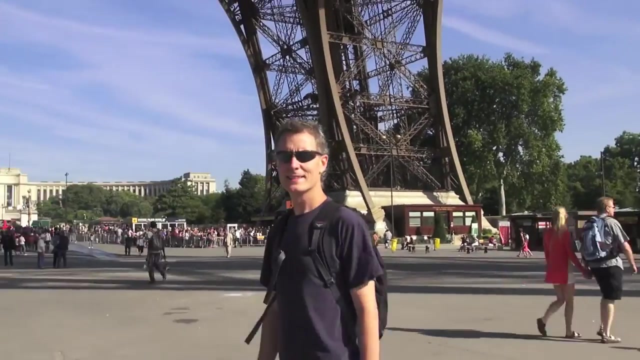 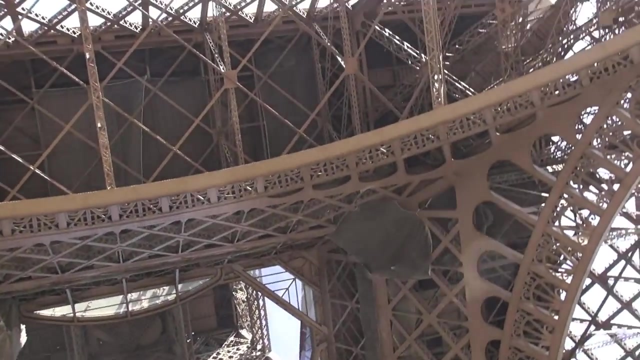 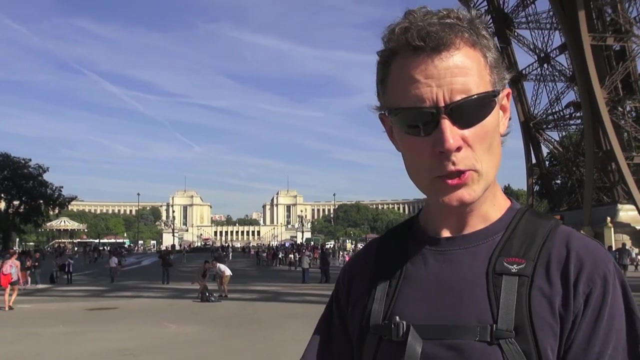 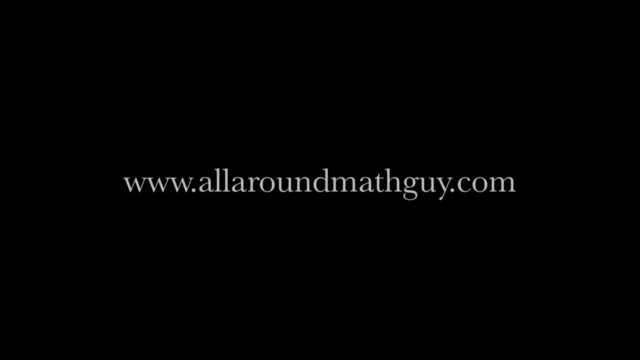 and look from right underneath it, though you pretty unbelievable when you're standing here. how big does that thing actually end? anyways, there's a pretty pretty good use of scale: how much bigger something is. Thanks for watching.